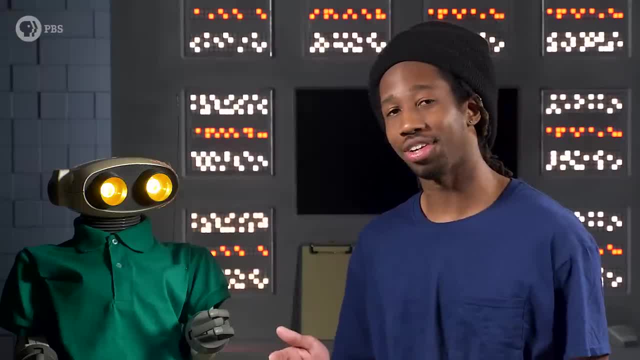 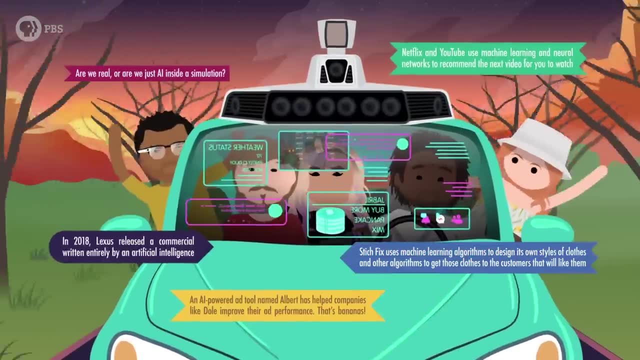 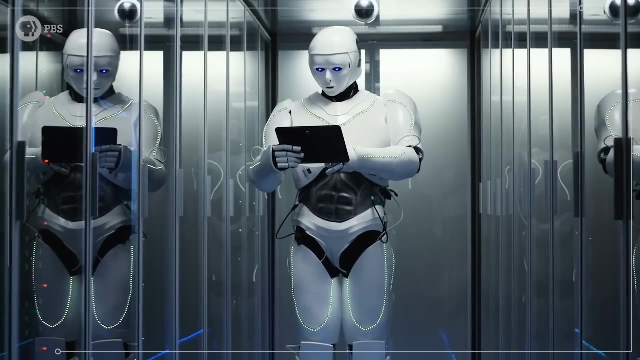 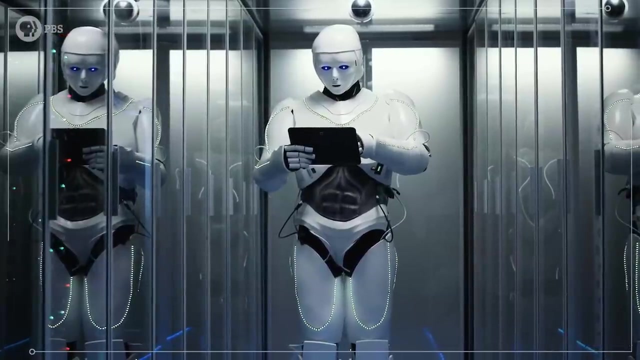 intelligence might be headed and our role in the AI revolution. we have to understand how we got to where we are today. If you know about artificial intelligence mostly from movies or books, AI probably seems like this vague label for any machine that can think like a human. Fiction writers like to imagine a more generalized AI, one that 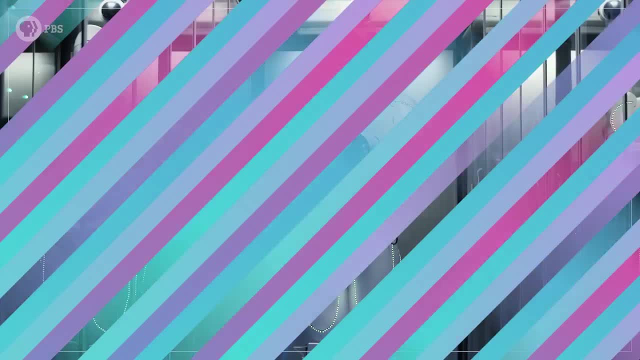 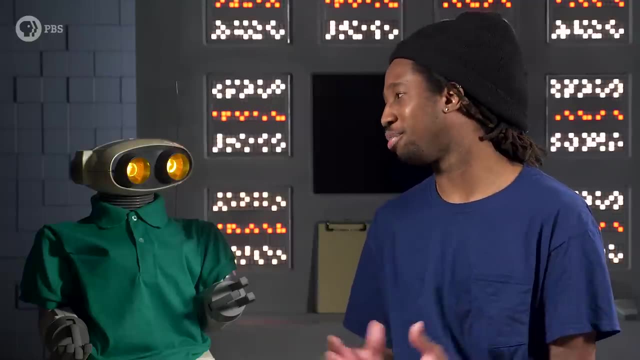 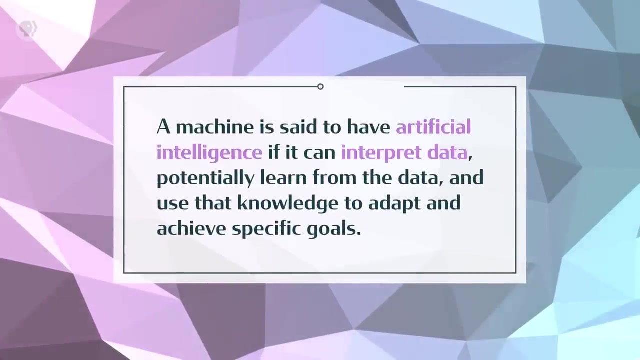 can answer any question you might have and do anything a human can do. But that's a pretty rigid way to think about AI and it's not super realistic. Sorry, John GreenBot, you can't do all of that. yet A machine is said to have artificial intelligence if it can interpret data, potentially learn. 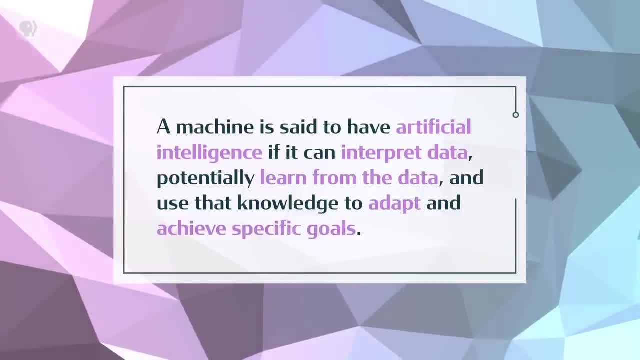 from the data and use that intelligence to do something. But AI is not a machine that's going to learn from the data and use that knowledge to adapt and achieve specific goals. Now the idea of learning from the data is kind of a new approach, but we'll get more. 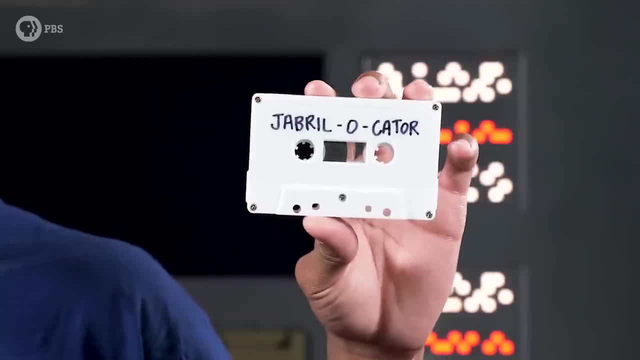 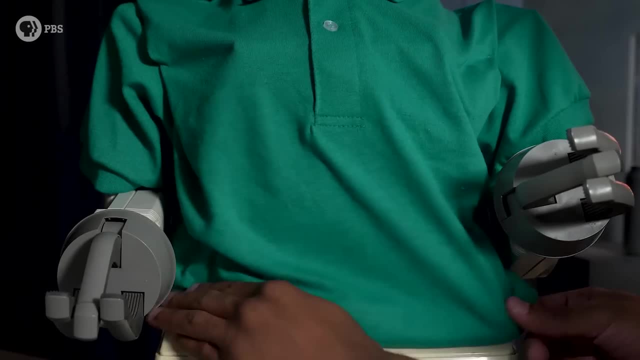 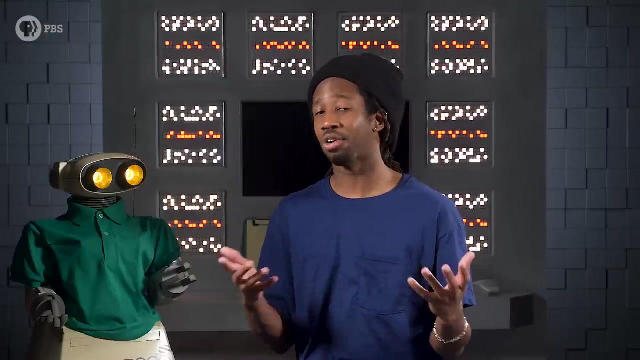 into that in episode 4.. So let's say we load a new program into John GreenBot. This program looks at a bunch of photos of me and some not of me and then learns from the data. Then we can show him a new photo, like this selfie of me here in the studio filming this. 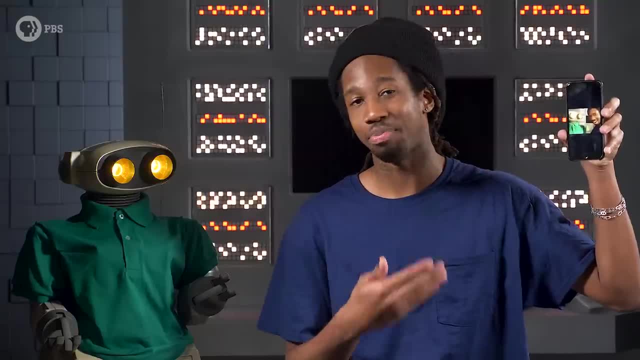 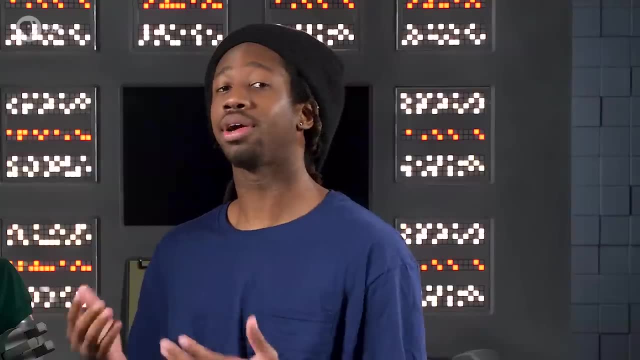 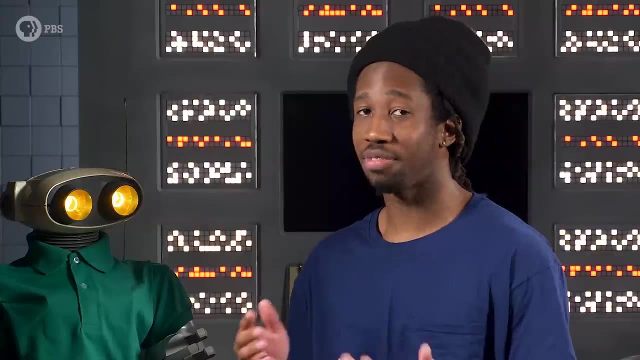 Crash Course video and we'll see if he can recognize if the photo is me. If he can correctly classify that new photo, we can say that John GreenBot has some artificial intelligence. Of course, that's a very specific input of photos and a very specific task of classifying. 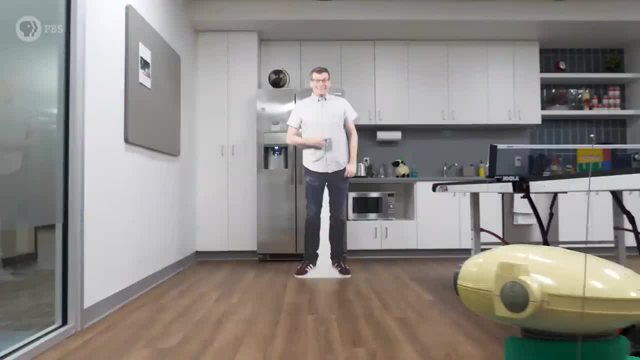 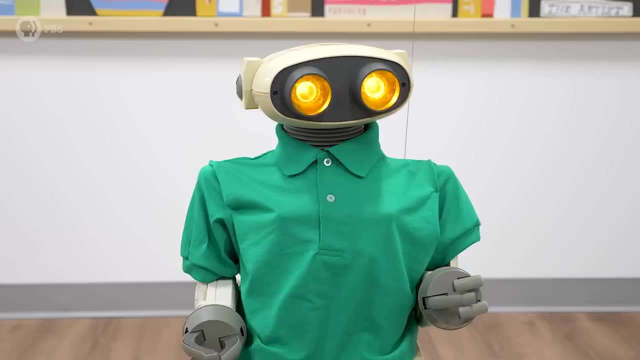 a photo that's either me or not me, And then we can show him a new photo, like this selfie of me here in the studio filming this Crash Course video, and we'll see if he can recognize if the photo is me Or just that program. John GreenBot can't recognize or name anyone who isn't me. 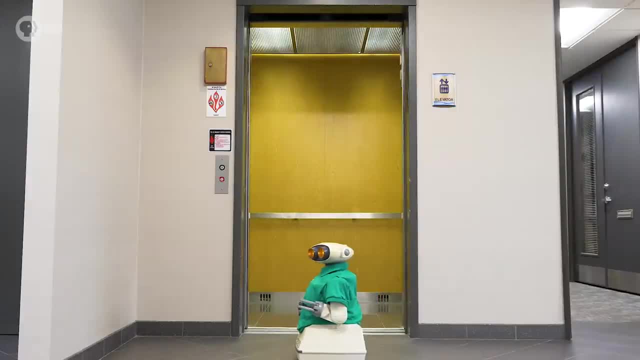 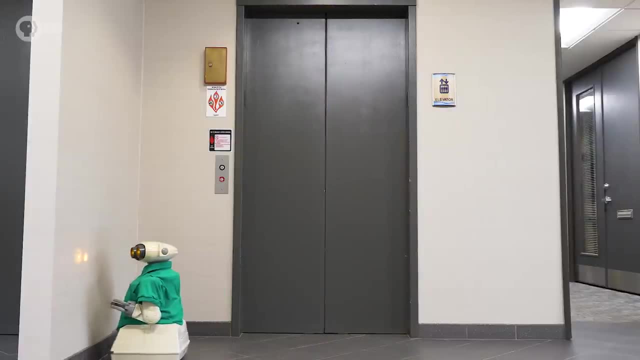 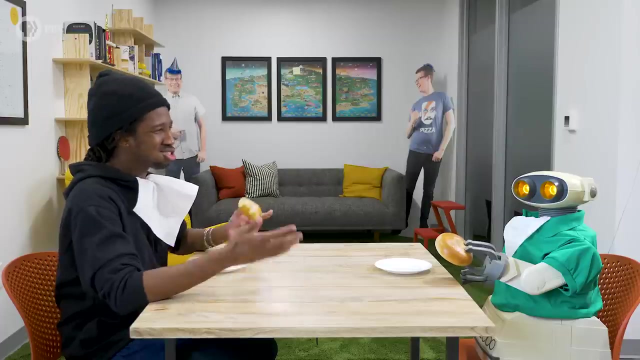 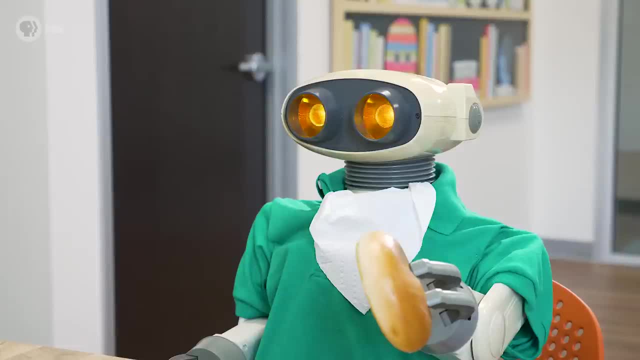 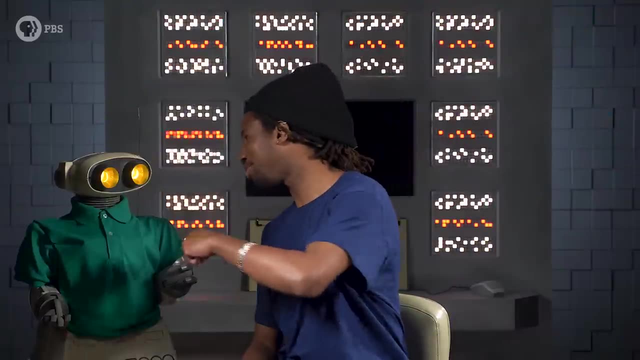 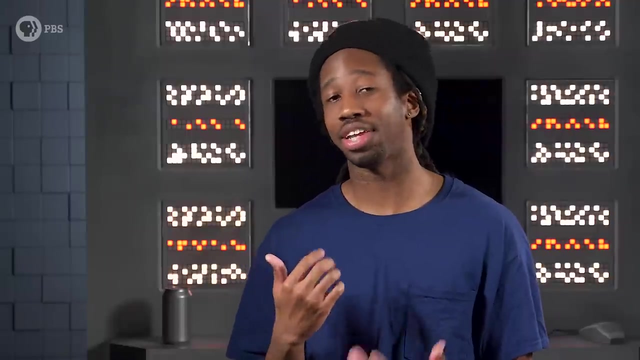 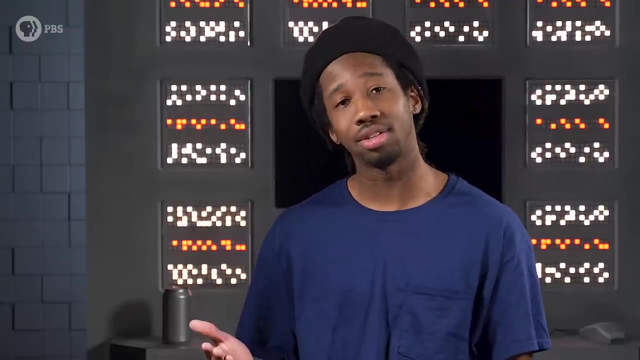 I don't get it. I just don't get it. I just don't get it. He can't do most things that humans do, which is pretty standard for AI these days, But even with this much more limited definition of artificial intelligence, AI still plays. 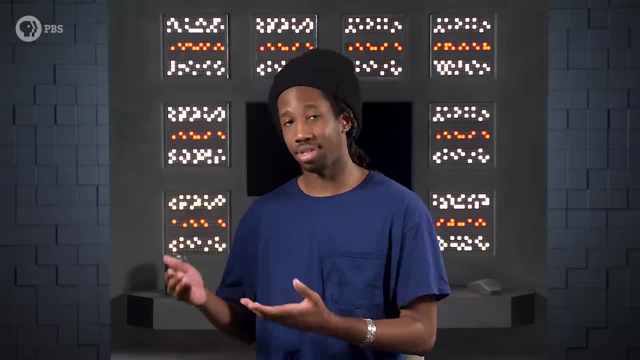 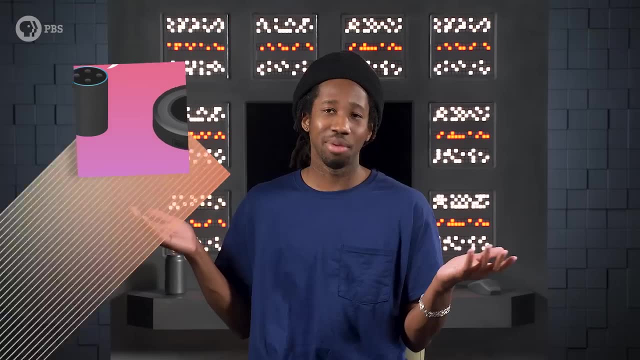 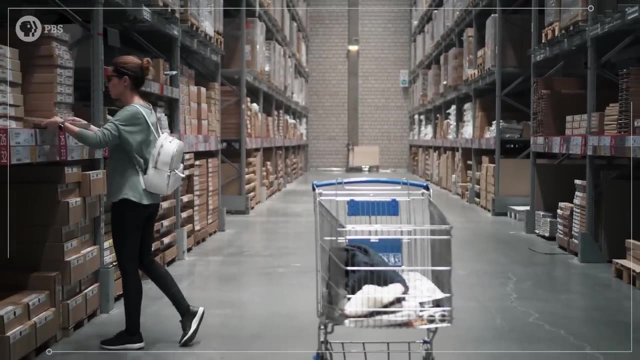 a huge role in our everyday lives. There are some more obvious uses for AI, like Alexa or Roomba, Which is kinda like the AI from science fiction, I guess, But there are also a ton of less obvious examples. When we buy something in a big store or online, we have one type of AI deciding which and 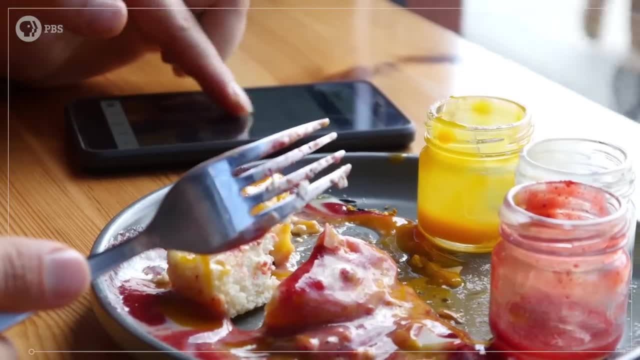 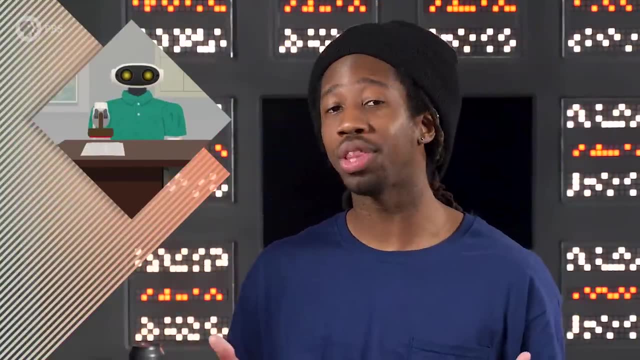 how many items to stock. And as we scroll through Instagram, a different type of AI picks ads to show us. AI helps determine how expensive our car insurance is or whether we get approved for a loan, And AI even affects big life decisions. 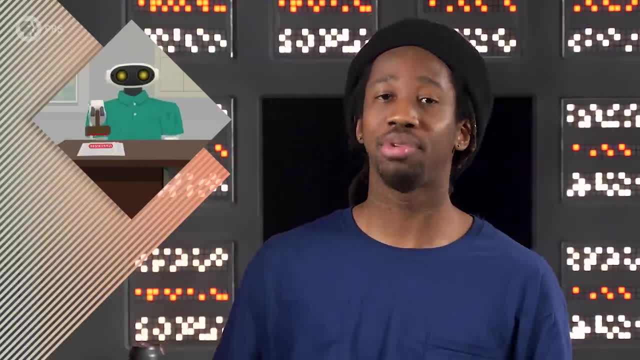 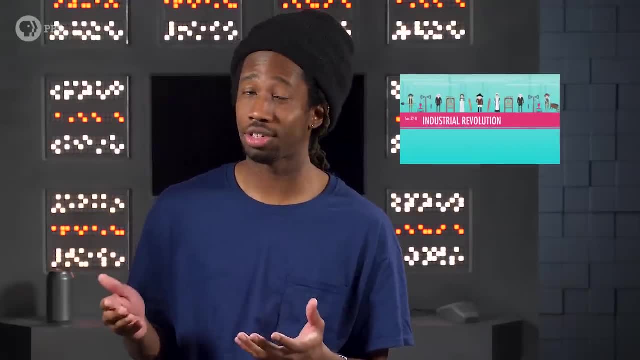 Like when you submit your college or job application. AI might be screening it before a human even sees it. The way AI and automation are changing commerce and jobs is sort of like the industrial revolution in the 18th century. This change is global. 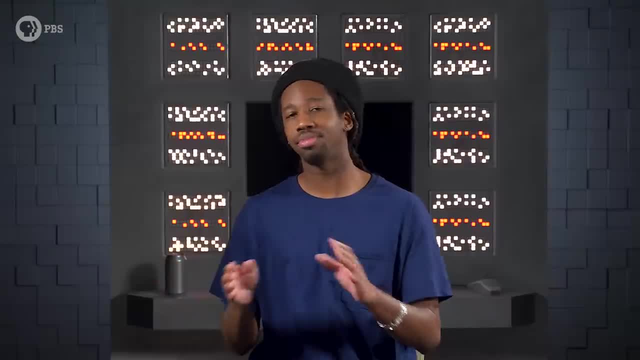 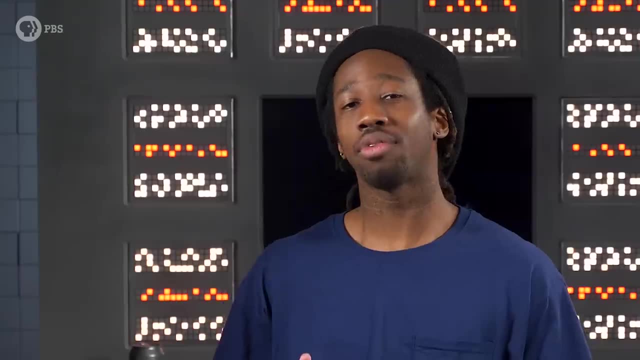 Some people are excited about it and others are afraid of it, But either way, we all have a responsibility to understand AI and figure out what role AI will play in our lives. The AI revolution itself isn't even that old. The term artificial intelligence didn't even exist a century ago. 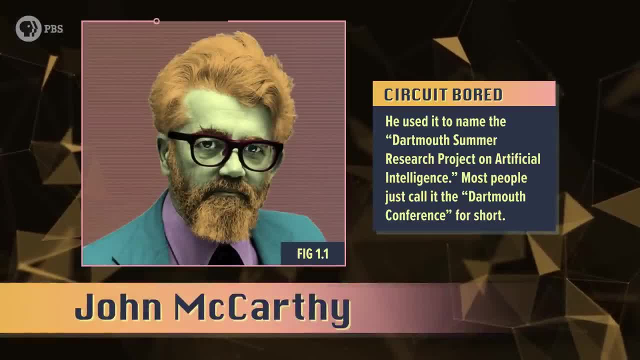 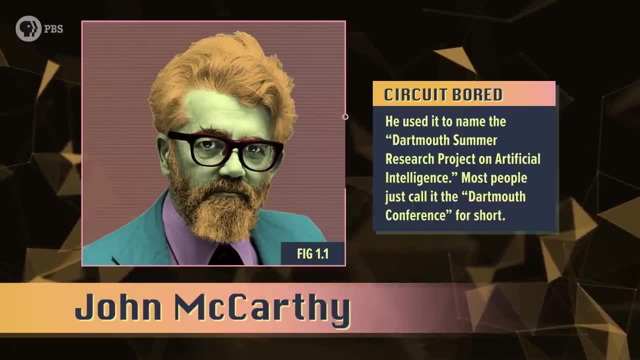 It was coined in 1956 by a computer scientist named John McCarthy. He used it to name the Dartmouth Research Project on Artificial Intelligence. Most people just call it the Dartmouth Conference for short. Now, this is way more than a weekend where you listen to a few talks and maybe go to 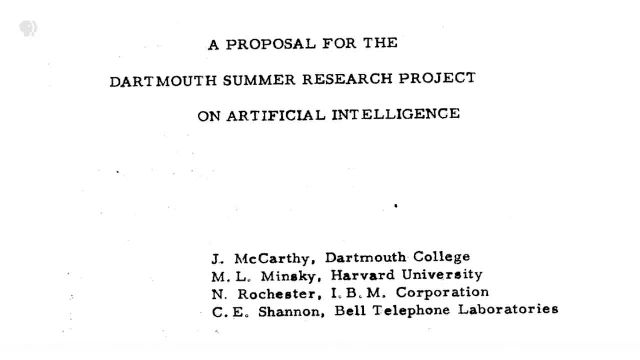 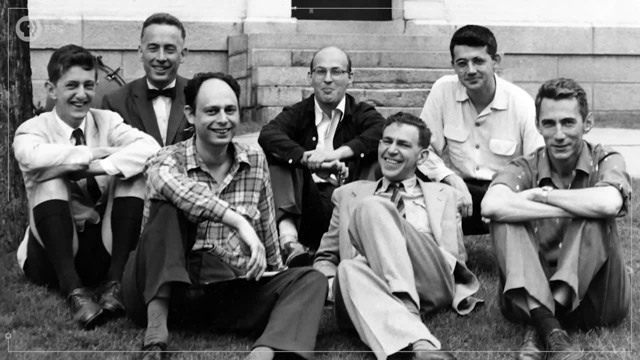 a networking dinner Back in the day, academics got together to think for a while. The conference lasted 8 weeks and got a bunch of computer scientists, cognitive psychologists and mathematicians to join forces. Many of the concepts that we'll talk about in Crash Course- AI, like artificial neural. 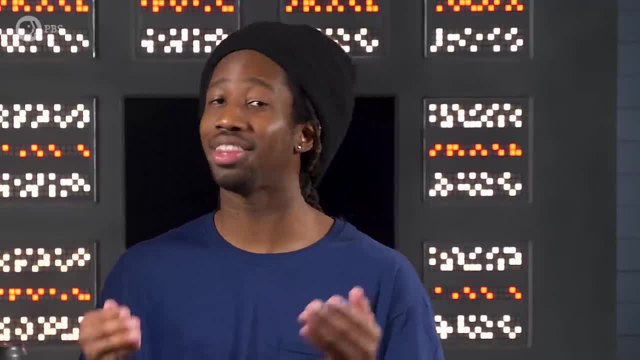 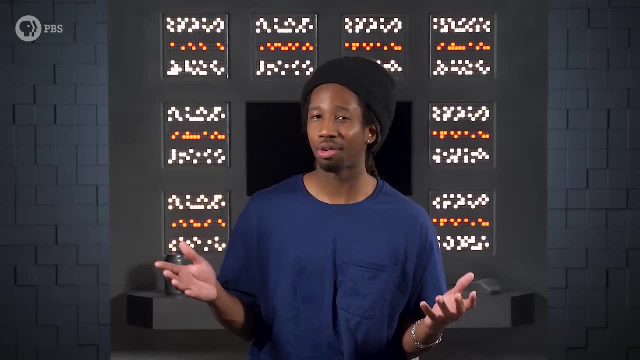 networks were dreamed up and developed during this conference and in the few years that followed. But because these excited academics were pretty optimistic about artificial intelligence, they may have oversold it a bit. For example, Marvin Minsky was a talented cognitive scientist who was a part of the 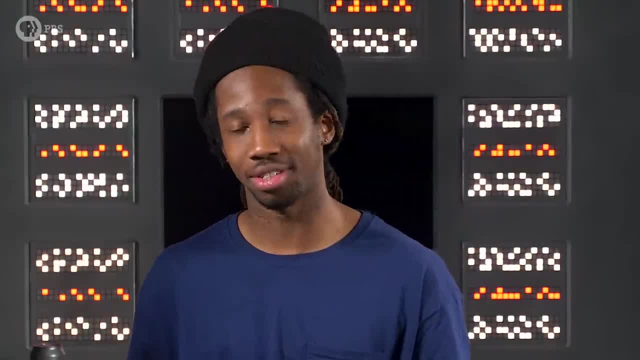 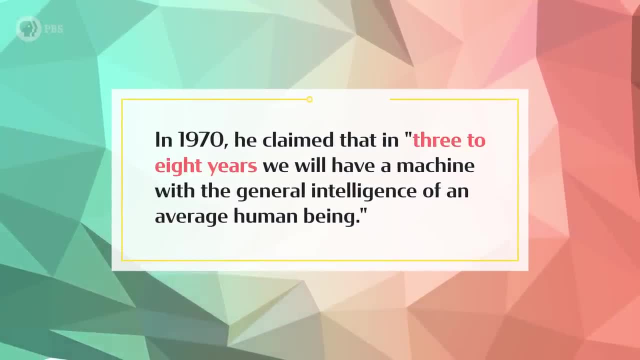 Dartmouth Conference, But he had some ridiculously wrong predictions about technology and specifically AI. In 1927, Minsky was a professor at the University of New York. In 1970, he claimed that in 3-8 years we will have a machine with the general intelligence. 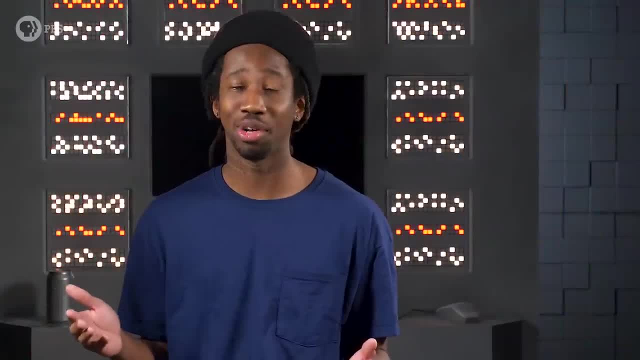 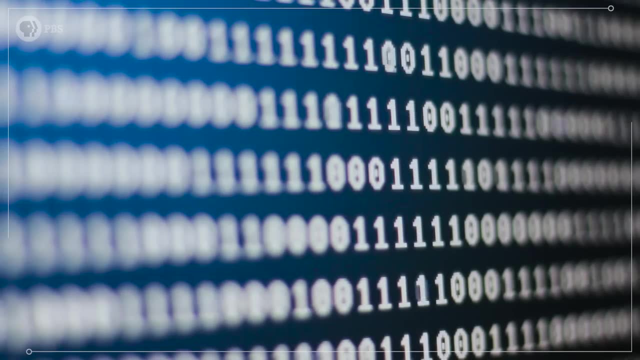 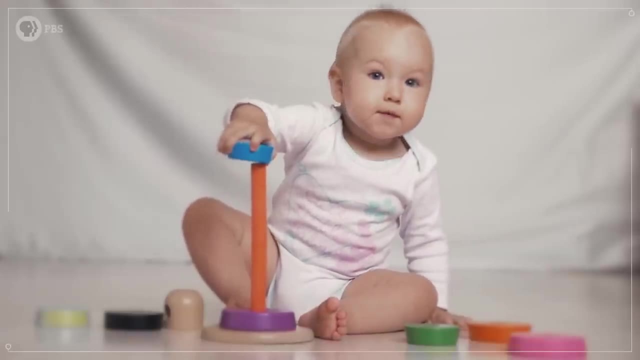 of an average human being, And sorry Marvin, but we're not even close to that now. Scientists at the Dartmouth Conference seriously underestimated how much data and computing power an AI would need to solve complex real-world problems. See, artificial intelligence doesn't really know anything when it's created. 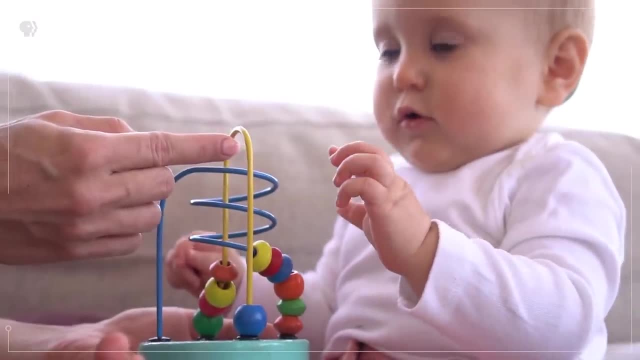 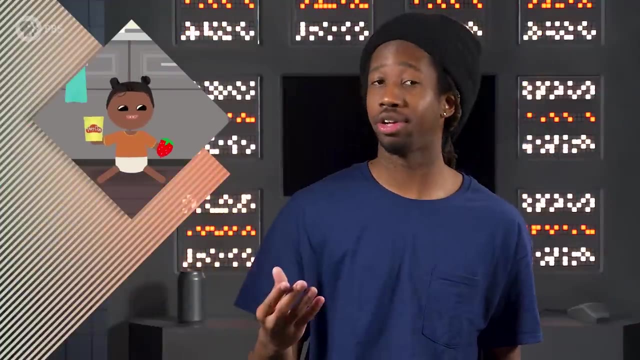 Kinda like a human baby. Babies use their senses to perceive the world and their bodies to interact with it, And they learn from the consequences of their actions. My baby niece might put a strawberry in her mouth and decide that it's tasty, And then she might put Play-Doh in her mouth and decide that it's gross. 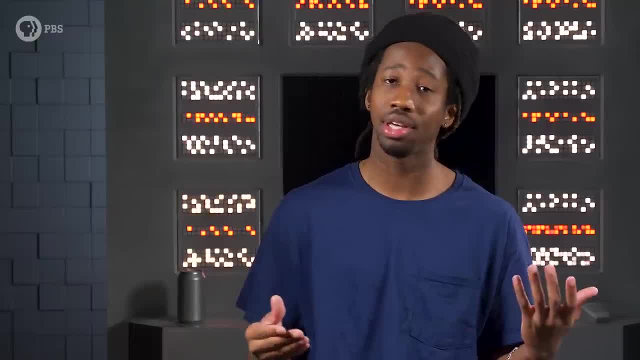 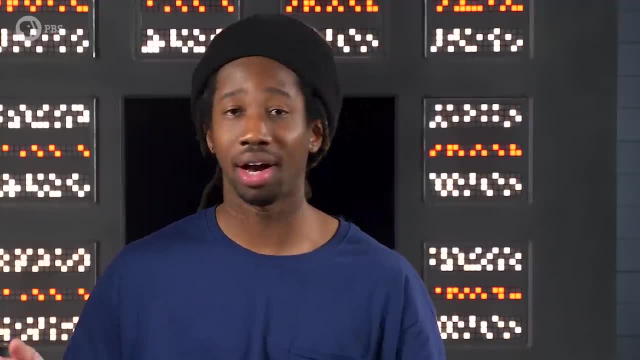 Babies experience millions of these data-gathering events as they learn to speak, walk, think and not eat Play-Doh. Now, most kinds of artificial intelligence don't have things like senses, a body or a brain that can automatically judge a lot of different things like a human baby. 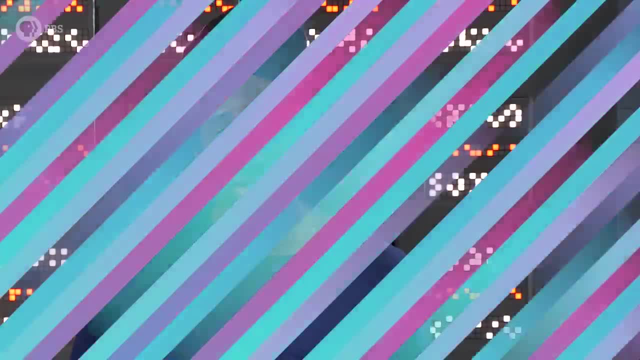 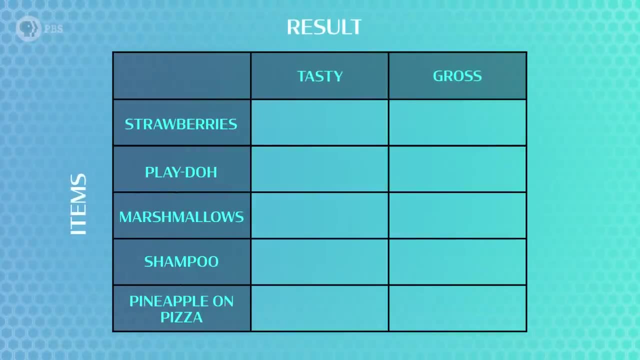 does. Modern AI systems are just programs and machines, So we need to give an AI a lot of data. Plus, we have to label the data with whatever information the AI is trying to learn, like whether food tastes good to humans, And then the AI needs a powerful enough computer to make sense of all the data. 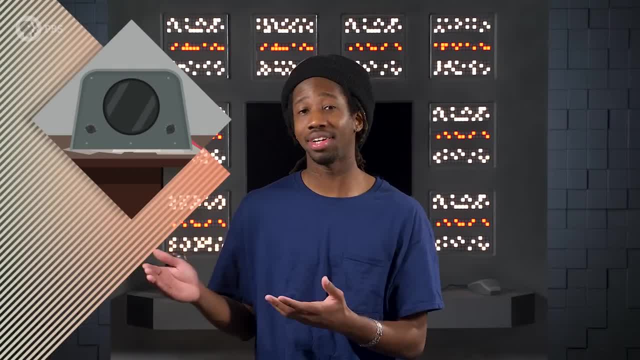 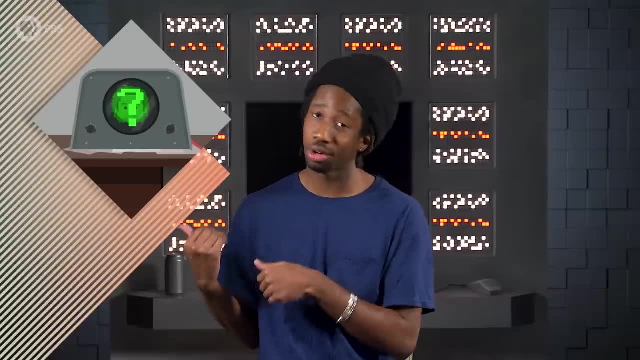 All of this just wasn't available in 1956. Back then, an AI could maybe tell the difference between a triangle and circle, but it definitely couldn't recognize my face in a photo like John Greenbott did earlier. So until about 2010 or so. 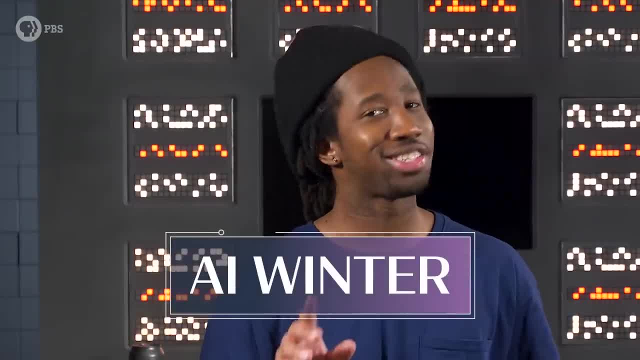 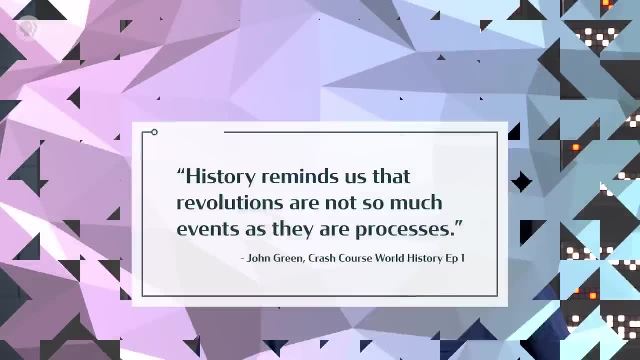 The world was basically frozen in what's called the AI winter. Still, there were a lot of changes in the last half a century that led us to the AI revolution. As a friend once said, history reminds us that revolutions are not so much events as 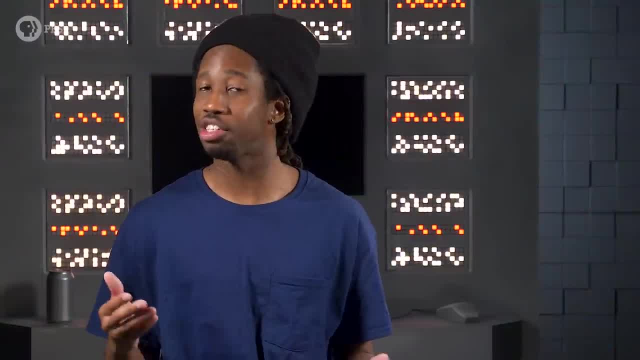 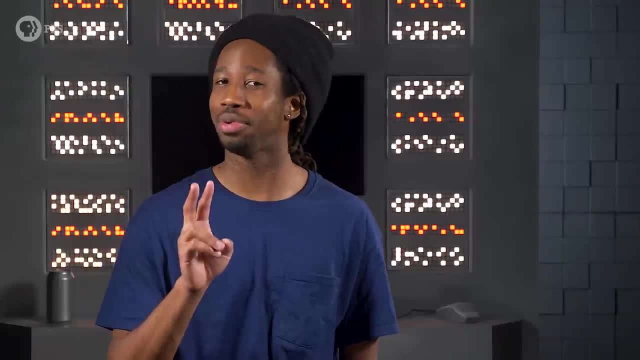 they are processes. The AI revolution didn't begin with a single event, idea or invention. We got to where we are today because of lots of small decisions and two big developments in computing. The first development was a huge increase in computing power and how fast computers 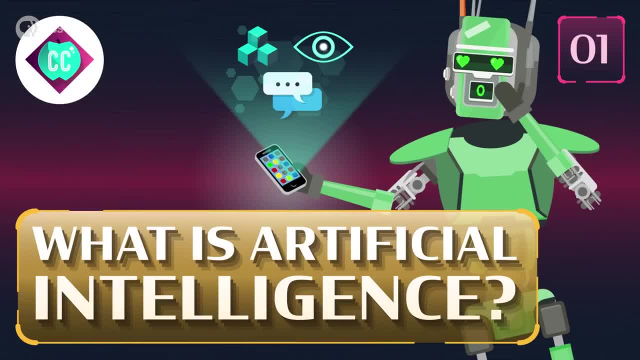 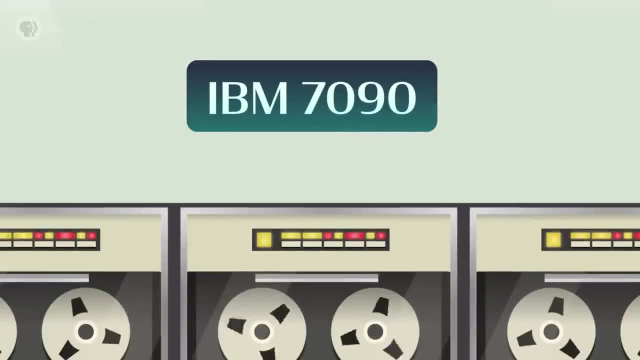 could process data. To see just how huge let's go to the Thought Bubble. During the Dartmouth Conference in 1956, the most advanced computer was the IBM 7090. It filled a whole room, stored data on basically giant cassette tapes and took instructions. 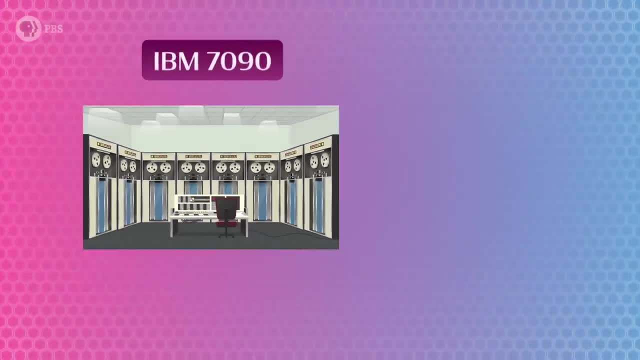 using paper punch cards Every second. the IBM 7090 could do about 200,000 operations, But if you tried to do that it would take you 55 and a half hours, assuming you did one operation per second and took no breaks. That's right, not even for snacks. At the time this was enough computing power to help with the US Air Force Ballistic Missile Warning System. But AI needs to do a lot more computations with a lot more data. The speed of a computer is linked to the number of transistors it has to do operations. 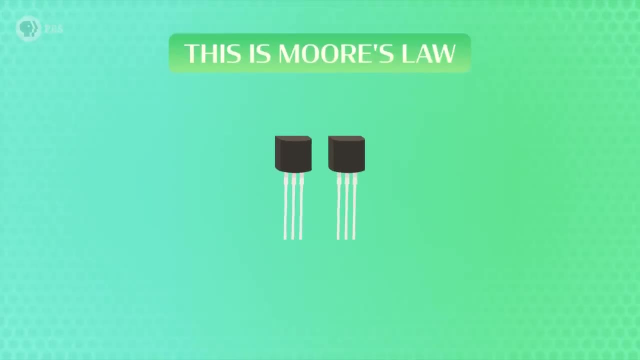 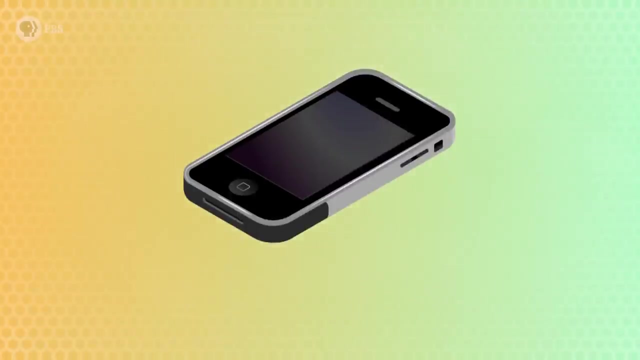 Every two years or so. since 1956, engineers have doubled the number of transistors, So computers have gotten much faster. When the first iPhone was released in 2007,, it could do about 400 million operations per second, But 10 years later, Apple says the iPhone X's processor can do about 600 billion operations. 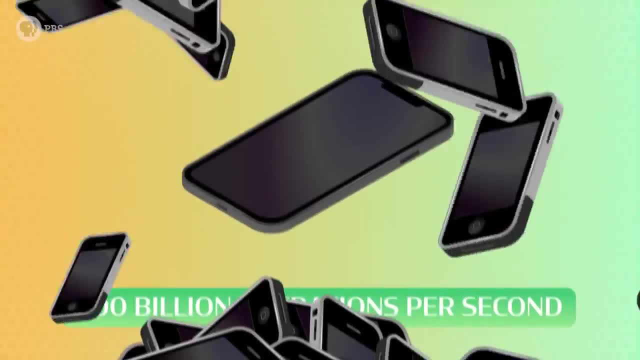 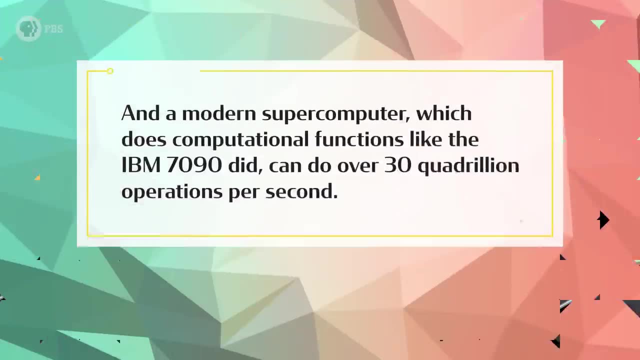 per second. That's like having the computing power of over a thousand original iPhones in your pocket For all the nerds out there. listen, you're right, it's not quite that simple. We're just talking about flops here, And a modern supercomputer which does kind of the same thing can do more than a thousand. 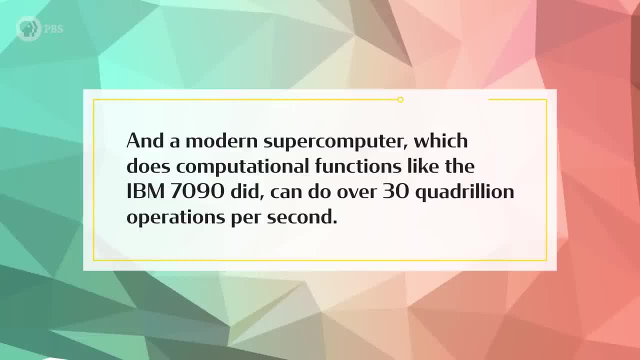 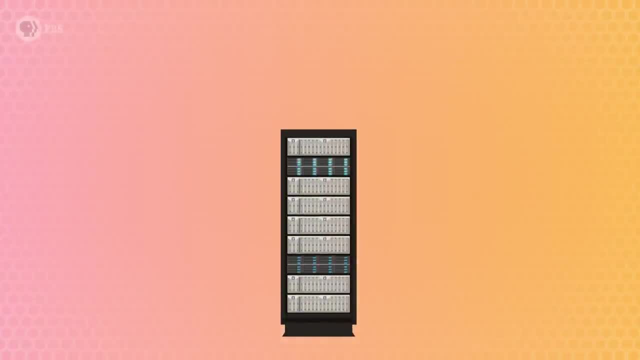 operations per second. Even the AI Z, which does computational functions, like the IBM 7 090 did, can do over thirty quadrillion operations per second. To put it another way, a program that would have taken a modern supercomputer one second. 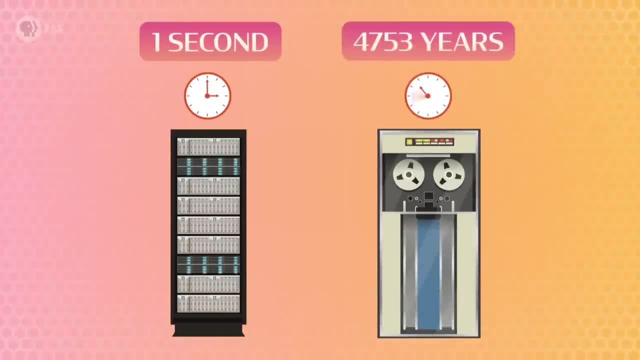 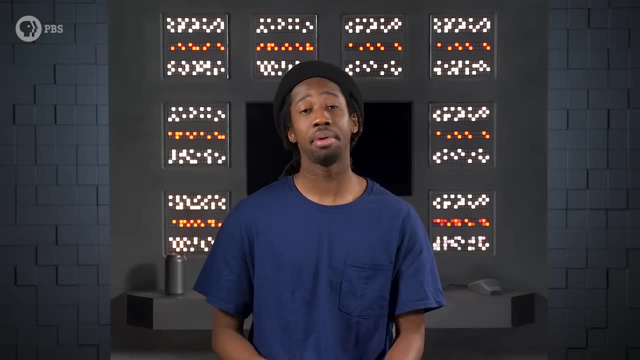 to compute would have taken the IBM 7 090. four thousand seven hundred and fifty-three years. Thanks Thought Bubble. So computers started to have enough computing power to mimic certain brain functions with artificial intelligence in 2005.. And that's when the AI 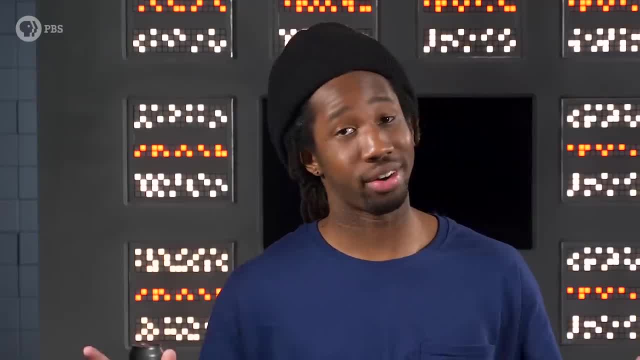 winters started to show signs of that. So that's my thought for it. Thank you for your time and I'll see you next time. But it doesn't really matter if you have a powerful computer, unless you also have a lot of data for it to munch on.